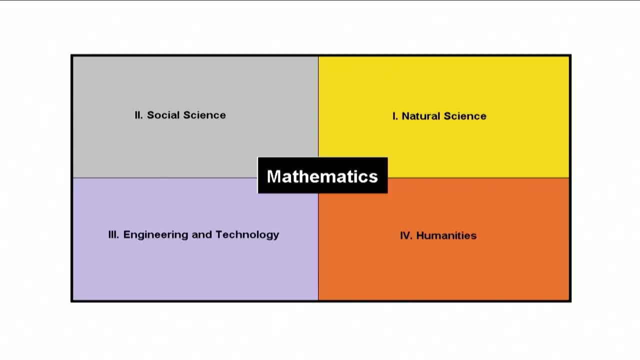 sciences and space science. You have the social sciences, where you'll find things like politics and economics, And then, of course, there's engineering and technology, where you'll find engineering fields: biomedical engineering, chemical engineering, computer engineering, electrical engineering, mechanical engineering, nuclear engineering and all the applications. 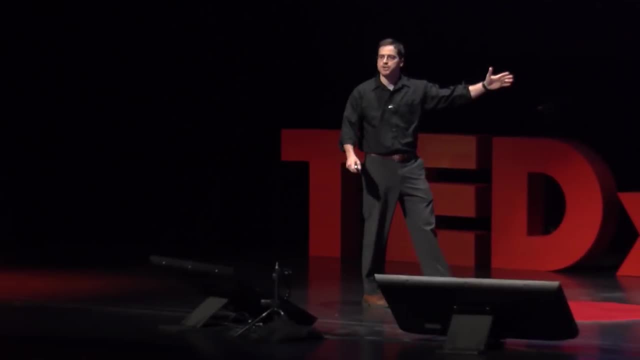 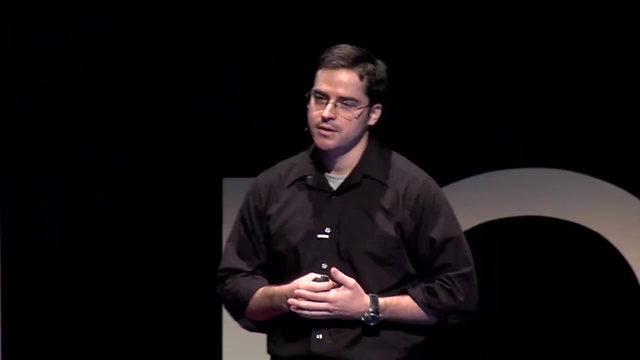 of technology, biotechnology, communications infrastructure and all of that. And last but certainly not least is the humanities, where you'll find things like philosophy, art and music. Now, math does show up in all of these disciplines, In some like physics. 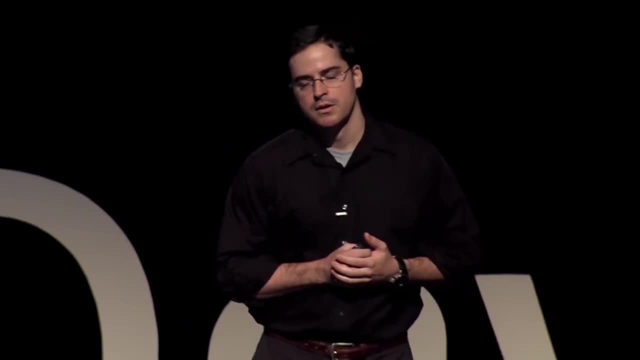 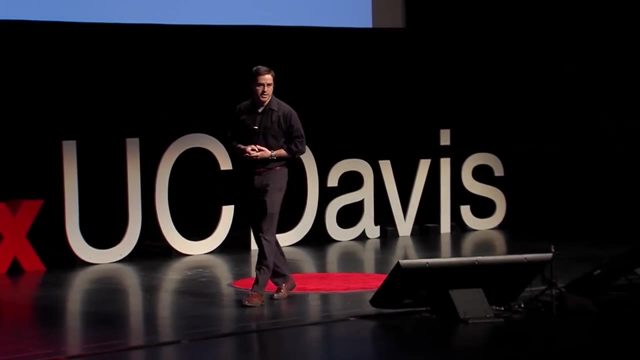 and engineering, the role of mathematics is quite pronounced and obvious, While in others, like in art and music, it's quite clear that the role of mathematics is quite pronounced and easy to understand. The role of mathematics is definitely somewhat more specialized and usually secondary. Nevertheless, math is everywhere And for that reason math is especially good. 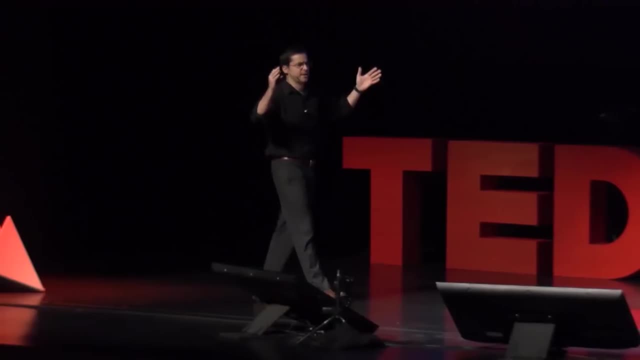 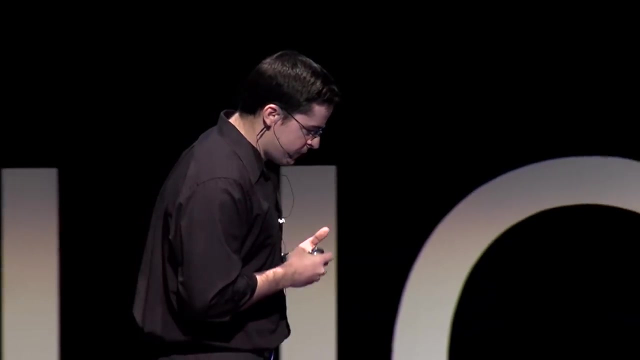 at making connections. How? How does math make connections? This is an excellent question. It's actually a question that's not easy to answer. I think for us now, in our time together, the best we can do is get a sense of what the answer to this question might look like. 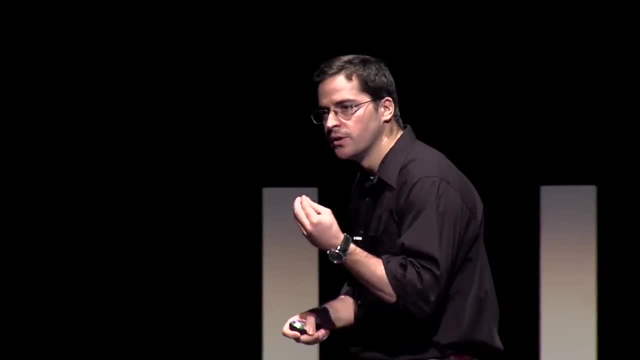 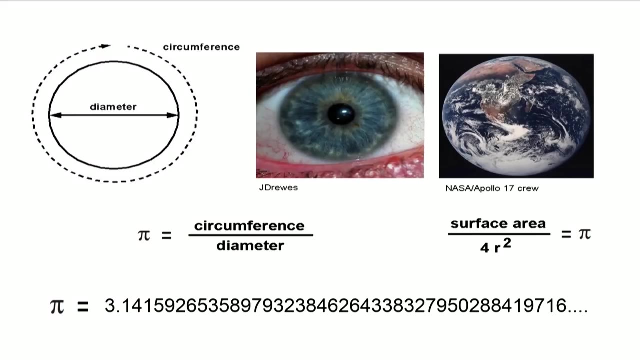 by examining some of the connections that mathematics can make through the lens of some mathematical ideas. Now, math is, of course, numbers, and perhaps the most famous number of all is the number pi. Pi was discovered because it represents a geometric property of the circle. It is the ratio of the circumference of every. 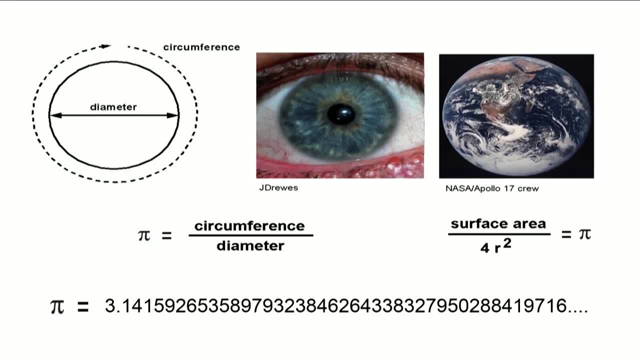 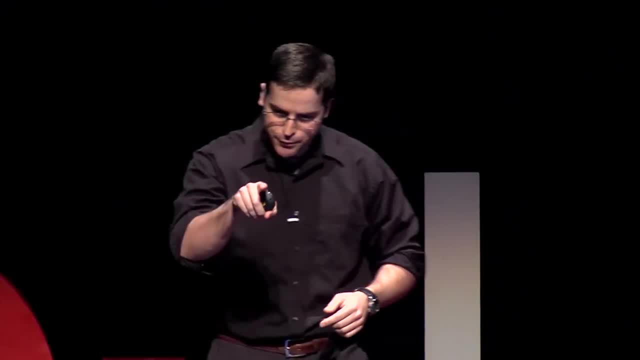 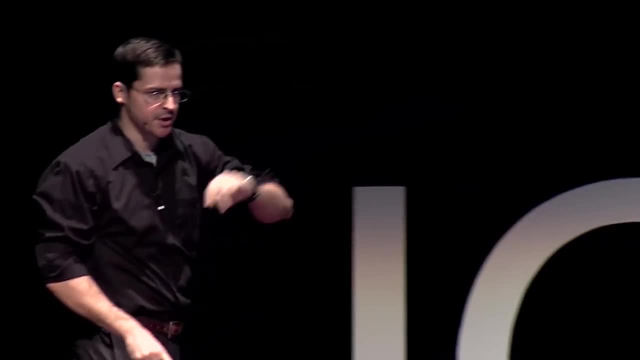 circle to its diameter, But nowhere in the world is anything a circle. Circle is a kind of pure mathematical idea, a construction from geometry that says you fix the center point and then you take all points that are equal distance from that center point. In two dimensions this construction produces a circle and 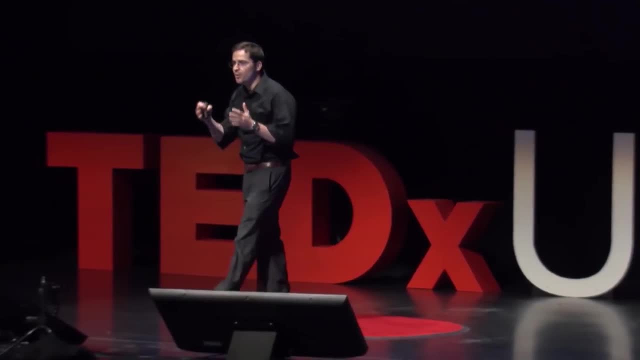 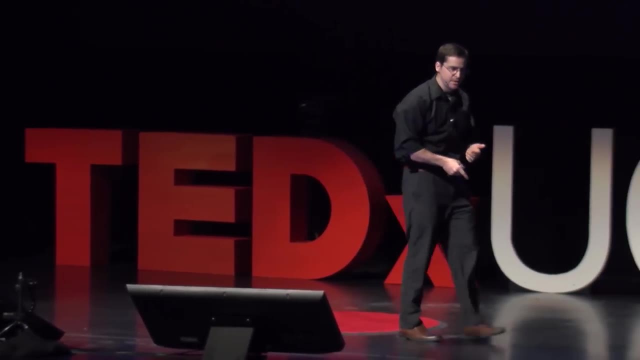 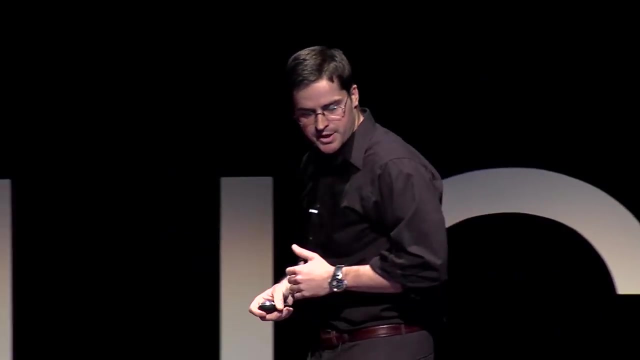 in three dimensions. the same construction produces a sphere, But nowhere in the universe is anything circle or sphere. This is a perfect, pure mathematical idea, and this world that we live in is imperfect, rough, atomized, moving, and everything is slightly askew. Nevertheless, the number pi has been. 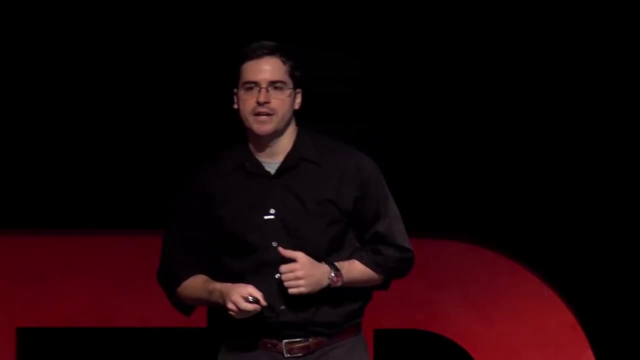 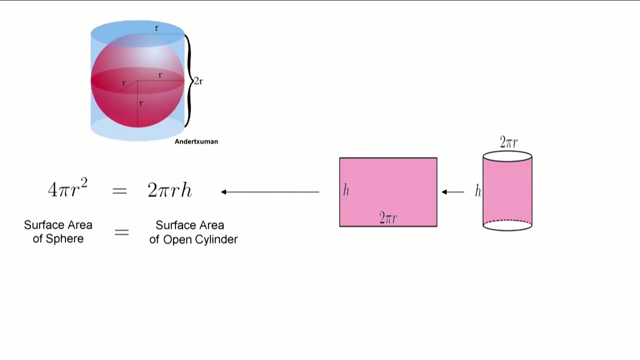 astonishingly useful to us throughout history. Let's go through some of that history together. Around the year 212 BC, Archimedes was murdered by a Roman soldier. His dying words were: do not disturb my circles. He wanted his favorite discovery put on his tomb: It's. 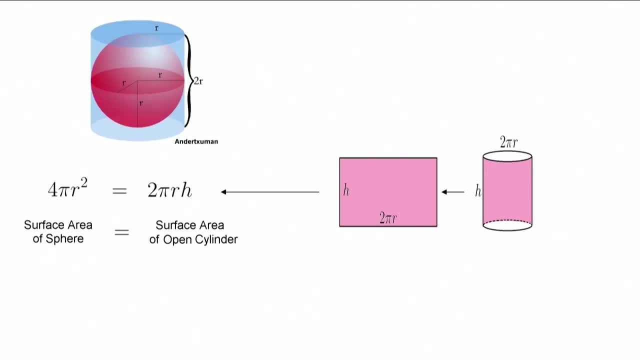 shown here. It says basically that the surface area of the sphere is equal to the surface area of the smallest open cylinder that can contain that sphere. Around 1620, Johannes Kepler discovered what he thought of as a harmony of planetary motion. Isaac Newton would later build on this. 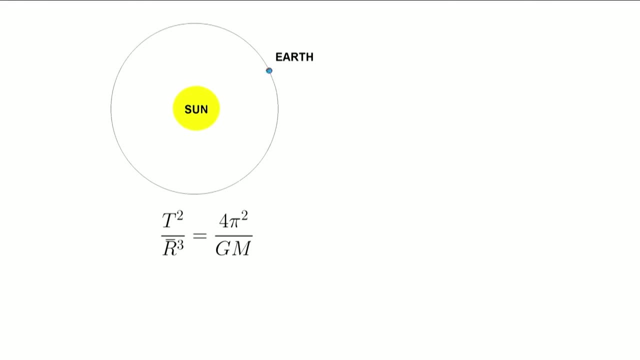 work shown here as Kepler celebrated third law of planetary motion. From sixteen to seventeen hundred, Christian Huygens, Galileo Galilei and Isaac Newton were early pioneers studying the pendulum. Shown here is a formula T for the period of the pendulum which tells us something about how long it. 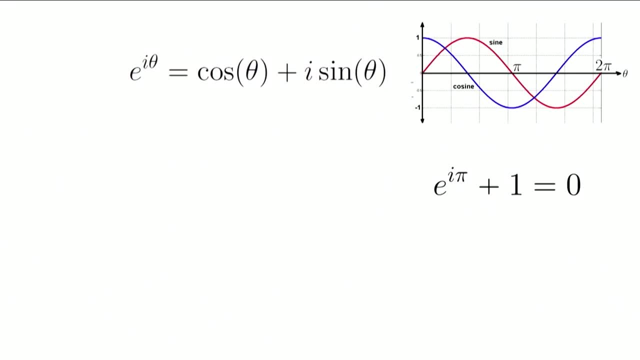 takes to swing back and forth. The greatest mathematician of the 18th century, Leonard Euler, is responsible for discovering this formula. e to the i theta equals cosine theta plus i sine theta. This formula provides a key connection between algebra, geometry and 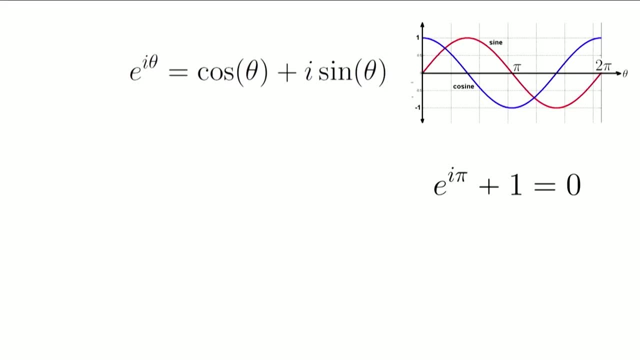 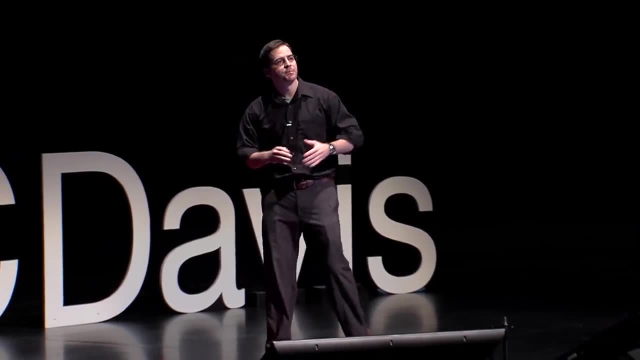 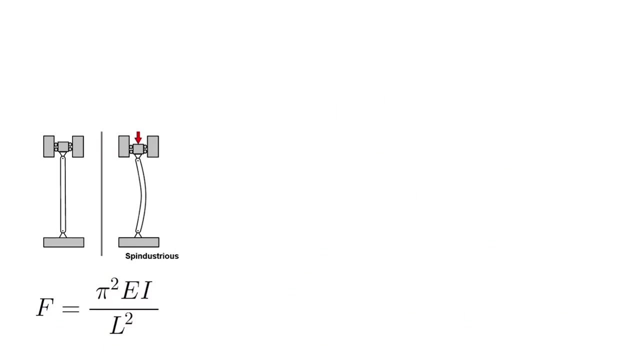 trigonometry. In the special case, when theta equals pi, it produces a relationship between arguably the five most important constants in all of mathematics: e to the i. pi plus one equals zero. Some people have called this the most beautiful formula in all of mathematics. Leonard Euler was also an engineer of some repute, and this formula- 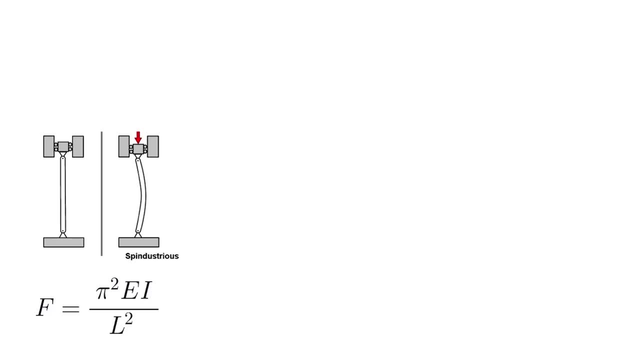 for f, the applied buckling force, that a column, as shown in the cartoon, will buckle under such an applied force as shown here. The greatest mathematician of the 19th century, Carl Friedrich Gauss, usually gets the credit for his work on what we call today the standard normal distribution. 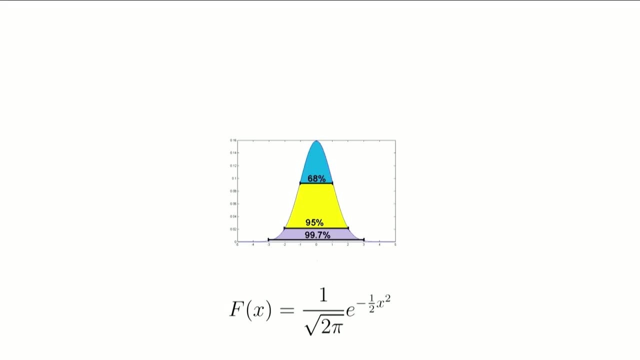 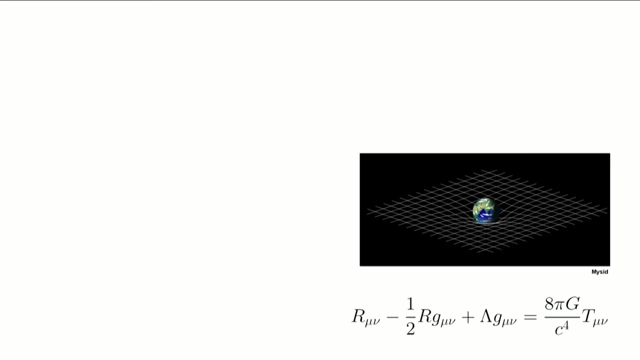 A staggering amount of real world data is distributed this way, according to what you might know as the bell curve of probability, And our tour of history ends in the 20th century with Albert Einstein and his famous theory of relativity. Shown here are Einstein's field equations: 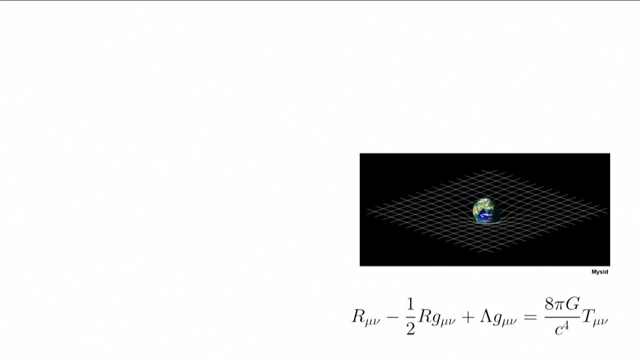 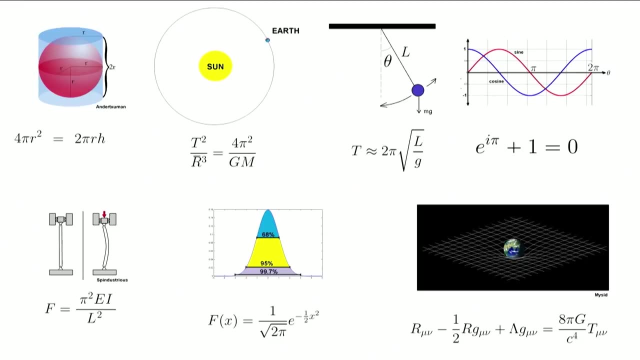 The difficulty to understand these equations is not to be underestimated. Now, that was too fast. I know That's a lot of information. There's no exam, no midterm, so just relax. Remember, we're trying to uncover connections. Now look at all of these. 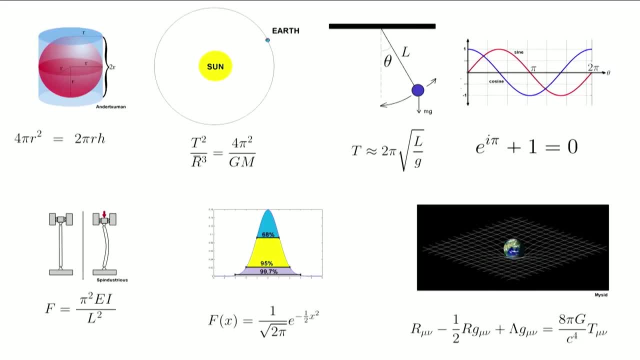 formulas, every one of them with pi in it, This number that was born from the geometry of the circle. And look at all of the physical phenomena, how different they all are And yet they share this common connection to this number, this geometric number from the circle. So when you 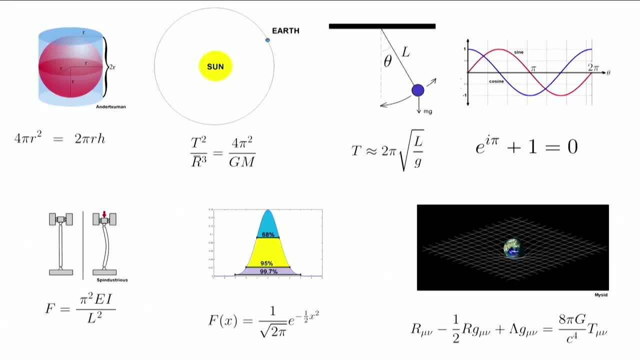 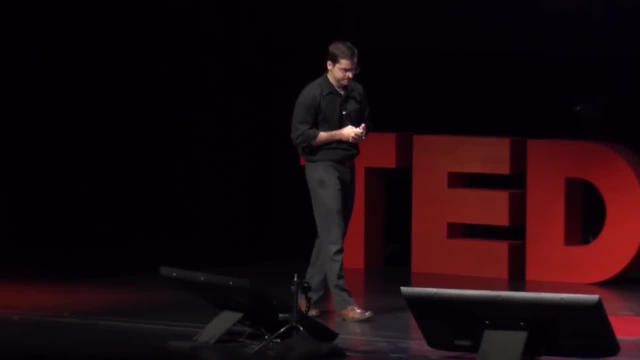 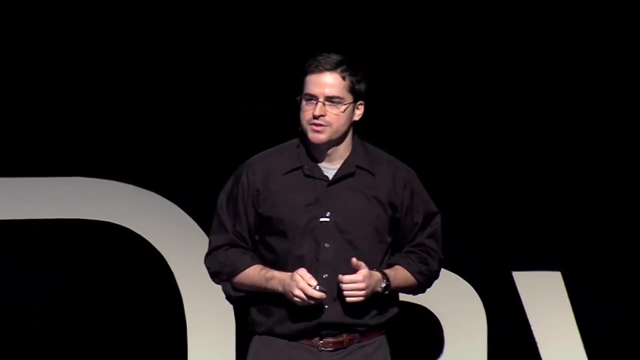 see a circle, when you see a formula and you see pi in it, you might think to yourself: maybe somehow, some way the circle plays a part in the derivation of this formula. Now, circle is just one geometric form and math is so much more, And so too is the world and the connections that 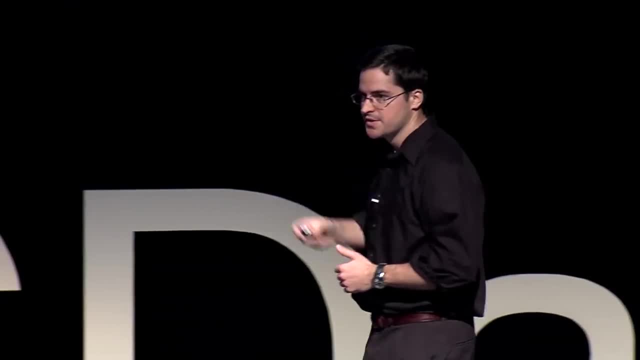 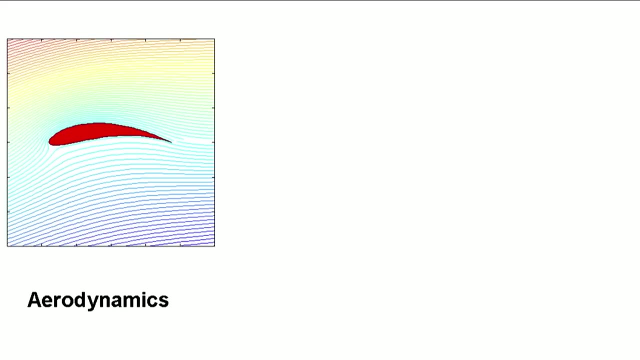 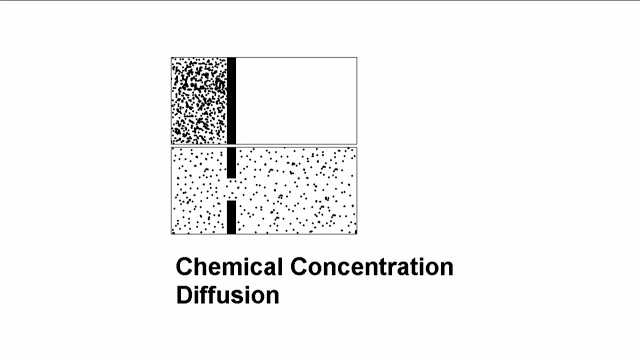 exist within it. Look here, this is an airfoil in 2D, like the cross-section of a wing, and the lines you see are like the air flowing over and under it. And here, at this experiment, this shows a gas initially compressed by a retaining wall into one side of a vessel, and then a hole is. 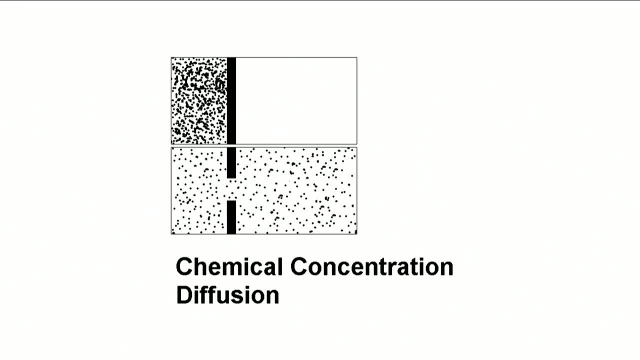 made in the retaining wall and the gas expands to fill the entire vessel until it reaches a constant And then it's compressed by a retaining wall into one side of a vessel and then a hole is made in the retaining wall into one side of a vessel and then a hole is made in the retaining wall. 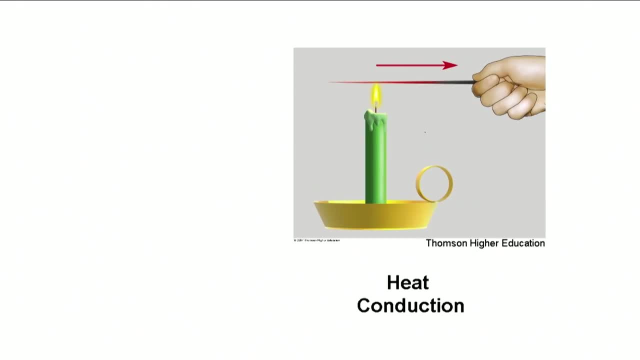 until it reaches a constant. And here, at this example, it shows a metal rod with a source of heat held under it, in this case a flame, And where the flame touches the metal at the point of contact, the heat will heat the rod and it will distribute along the rod until it reaches a 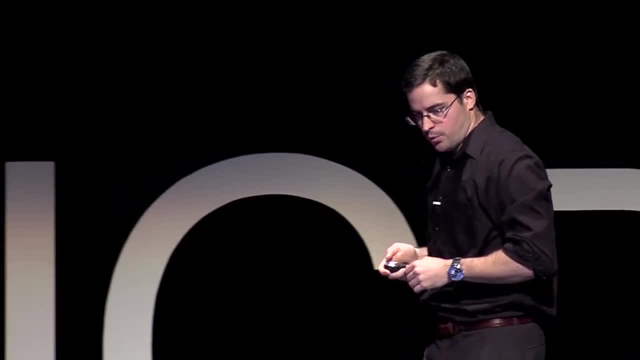 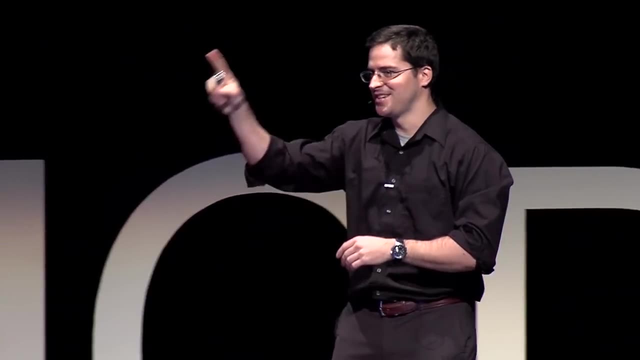 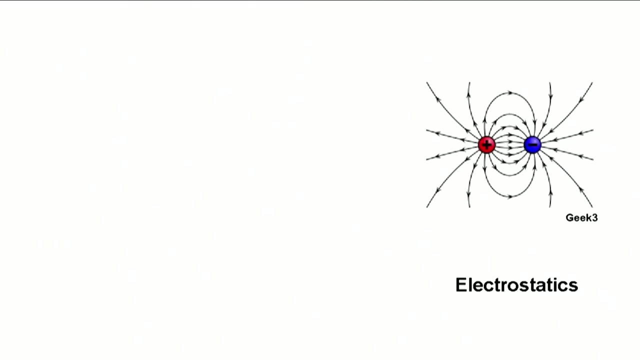 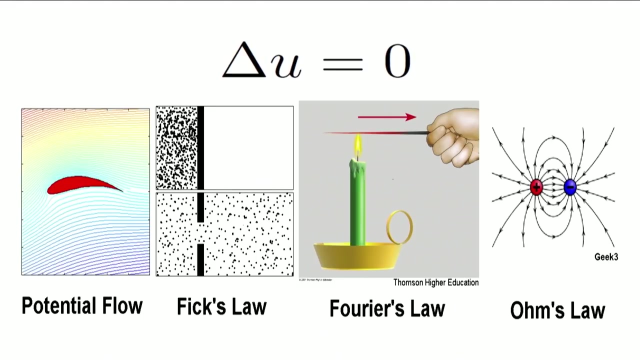 kind of thermal equilibrium, And it would not do. it would not do to have all of this science without electricity making an appearance. Shown here are the potential lines in an electric field which give us the paths that electrons will take, going from positive to negative charge. Now, all of these examples are very different to our. 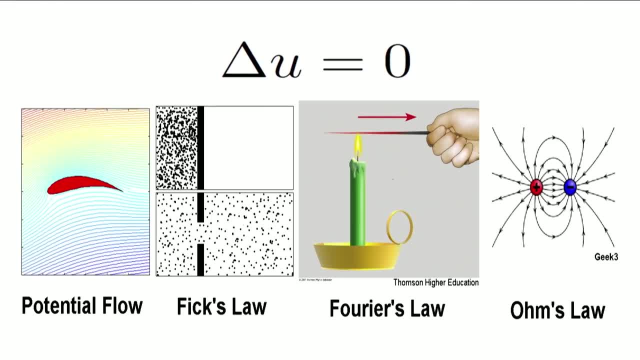 five senses. So different, in fact, that in science we give them all a different name. That's potential flow, Fick's law of chemical concentration, diffusion, Fourier's law of heat conduction and Ohm's law of electrical conductance. But in another kind of 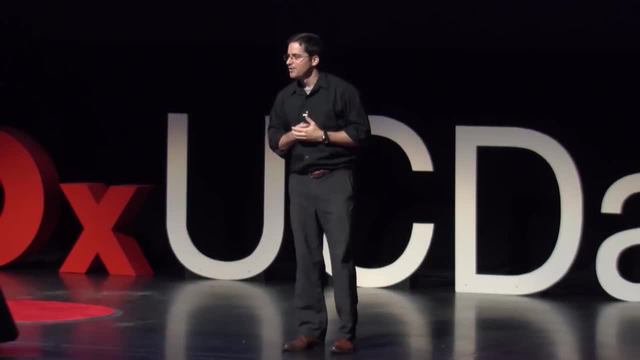 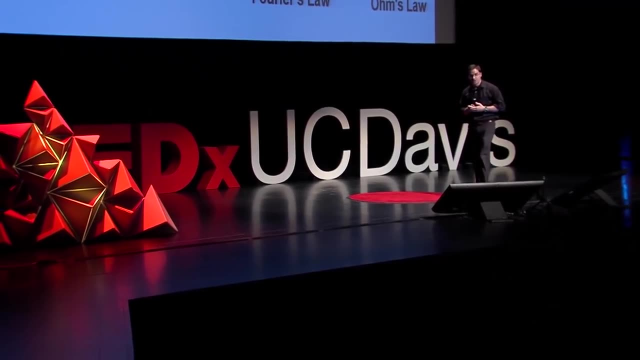 way, in a math kind of way. they're all very similar, So similar in fact, that in mathematics we give them all the same name. Laplace's equation, That's not triangle U equals zero, That's Laplacian of U equals zero. And what? 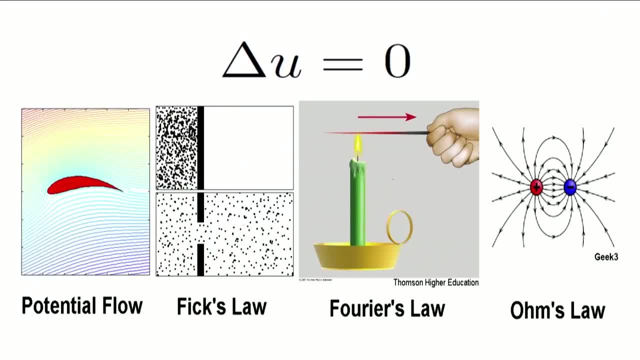 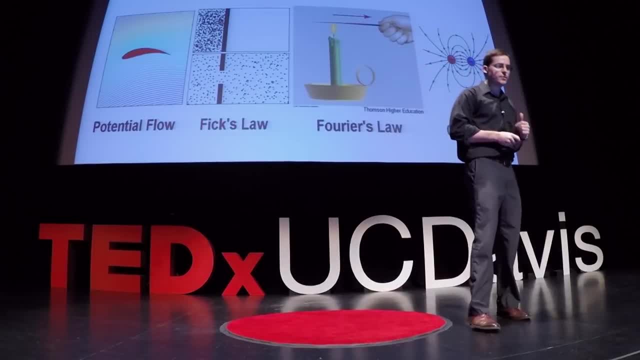 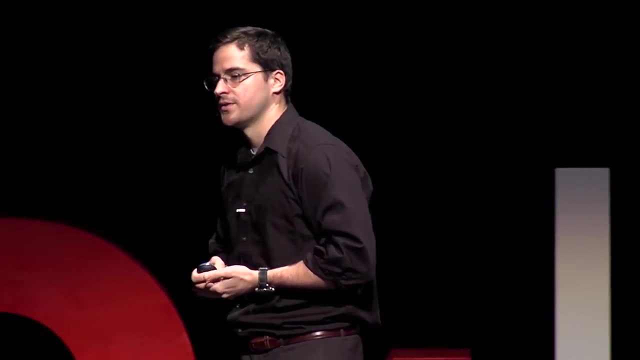 changes for the mathematician is: U can be potential and U can be chemical concentration and U can be heat and many other physical quantities that this equation can be used to describe from nature. You see, in mathematics not only do we have numbers and we have geometry, but we also have equations. 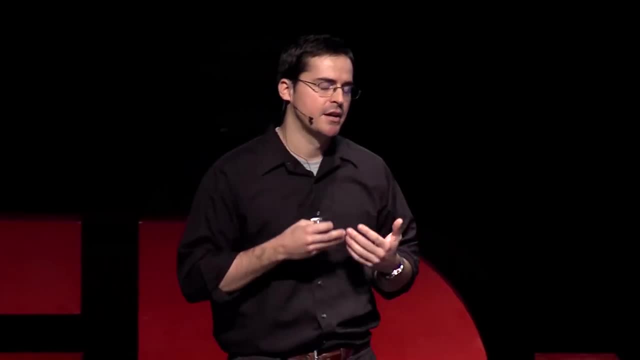 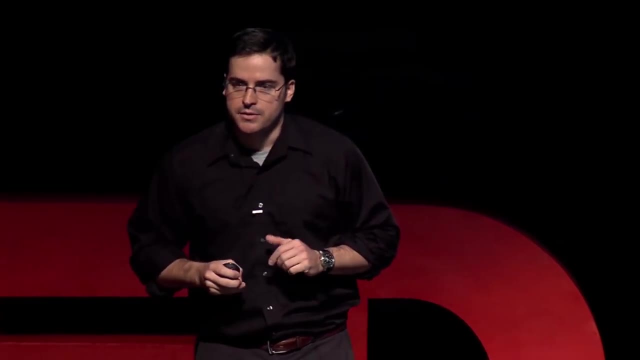 And when we compare the equations of things, this gives us yet another way in which we can describe things, in which things can be connected. Now, the connection between all of these science problems is calculus, and you should see that calculus is essential and foundational to modern computational. 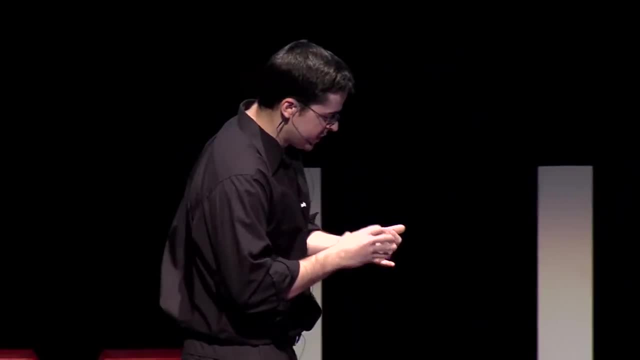 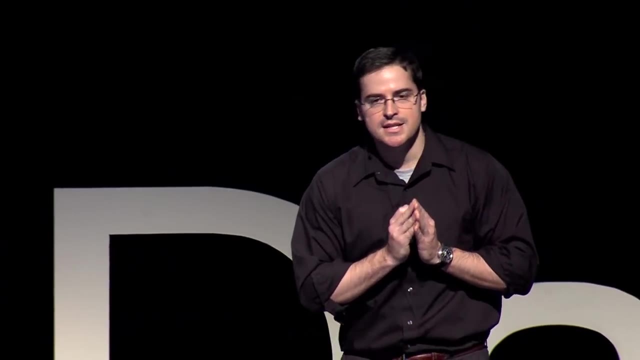 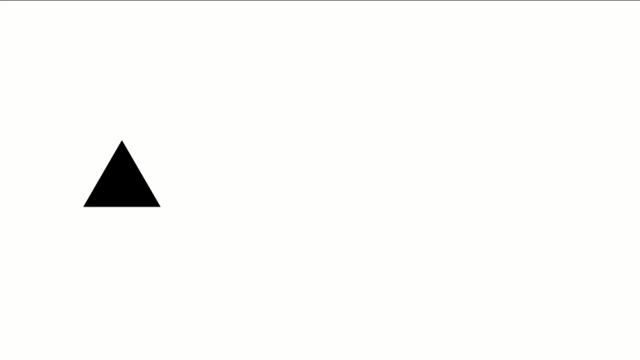 science. Now we've seen something about numbers and geometry and equations, but let's put it all together, because that's math, and let's see an application of mathematics. I want us to go through a construction here. This is what we'll call the first generation. 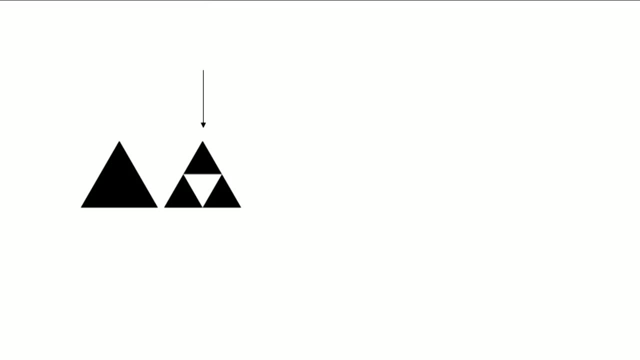 This the second generation. Look at the pattern: what happens to positive and negative space? And then the third generation, And so you see a pattern. start to develop Now in your mind. decide what the fourth generation should look like. Is this your expectation? And then the fifth generation, And then the fifth. 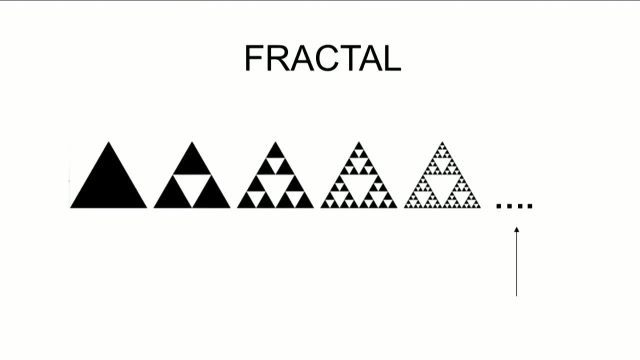 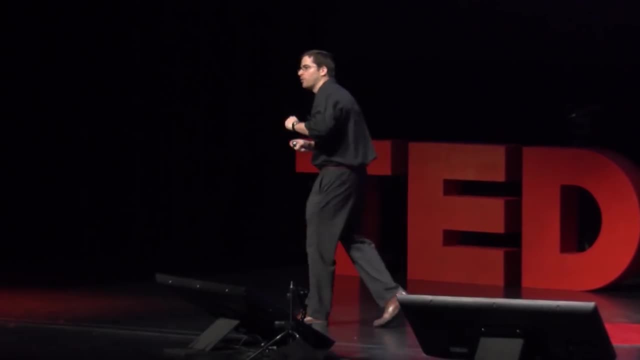 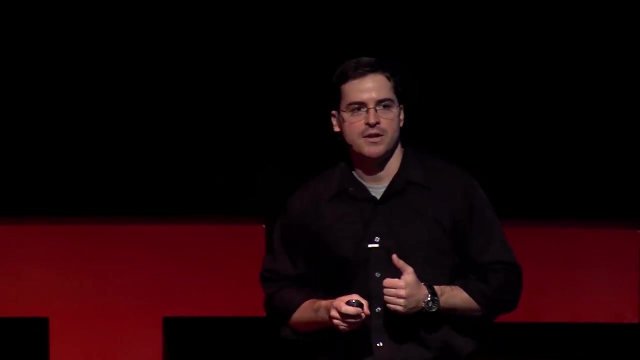 In fact, this is a famous fractal. It's the Sirpinski triangle. The fractal has never even been constructed in all of human history. It's never been completed. it can't be completed. It never terminates. When you see a fractal with your mind, you never see all of it. You. 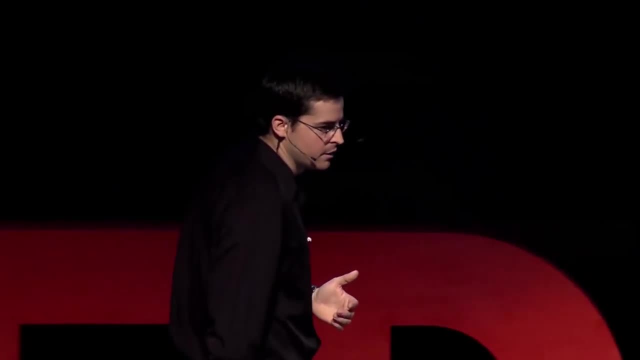 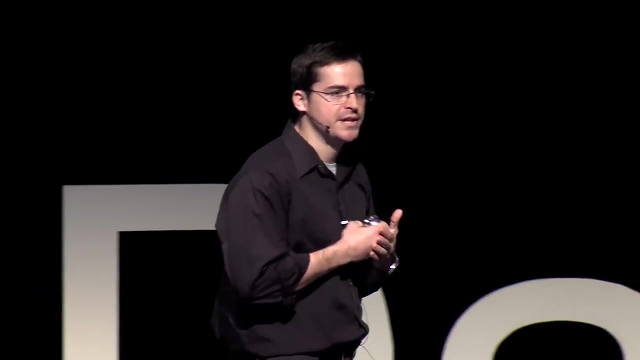 only get the sense of it Now. appreciation powers of fractals really took off in the 1970s after Benoit Mandelbrot's work, and part of the reason for the late bloom of this idea was that it really took the aid of the modern computer. 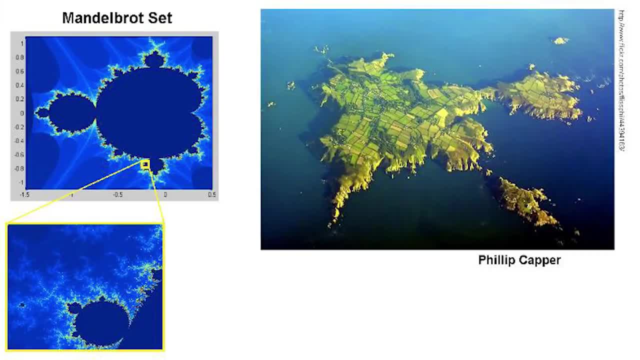 to properly compute and visualize this type of tremendous geometric complexity. Shown here at the top is the famous Mandelbrot fractal and notice there is a zoom up of a tiny segment of the fractal, magnified, so you can see it and just look at the complexity of that region. 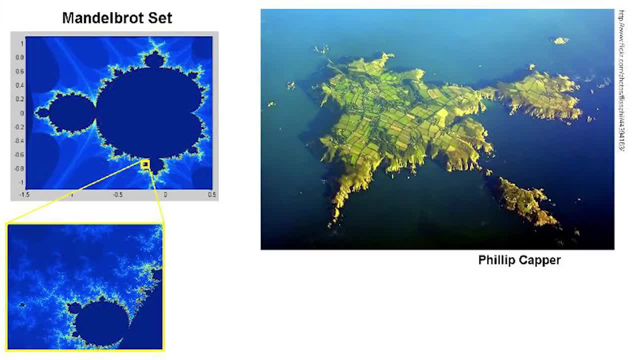 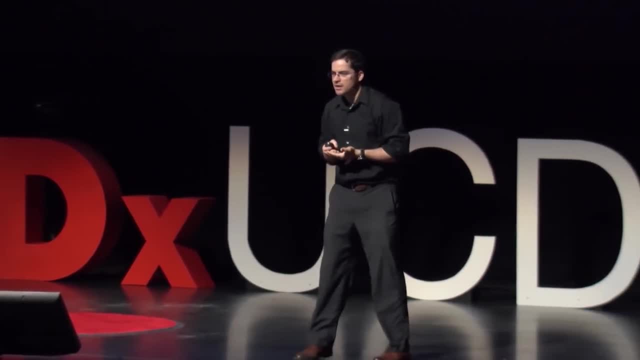 and if we zoom in there, in magnifying, no matter how much we zoom in to the fractal, the complexity will never diminish. This is not an easy thing to understand. This geometry is so complicated it is unclear if it has any equivalent in the natural world. and yet 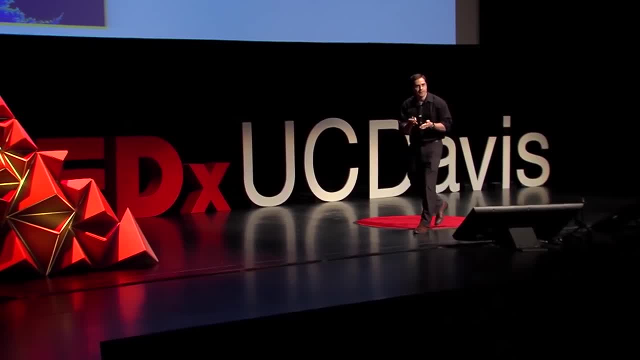 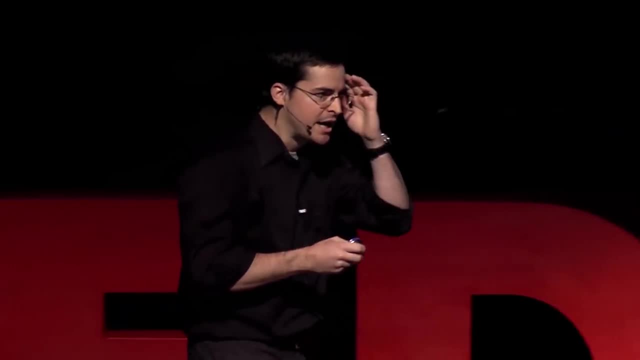 once people became aware of the existence of this kind of object, they started to see examples of it in applications everywhere. This is a kind of Baader-Meinhof phenomenon, where your mind becomes primed for knowledge and then, when you go out and look after learning. 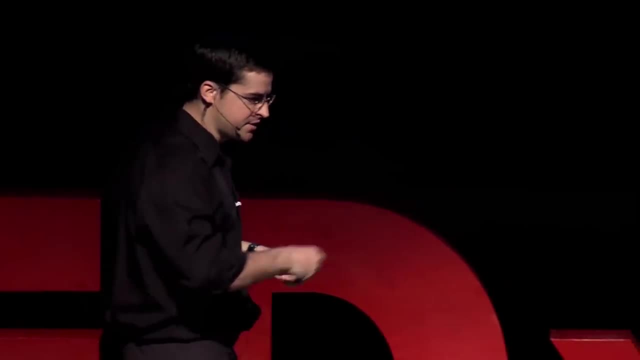 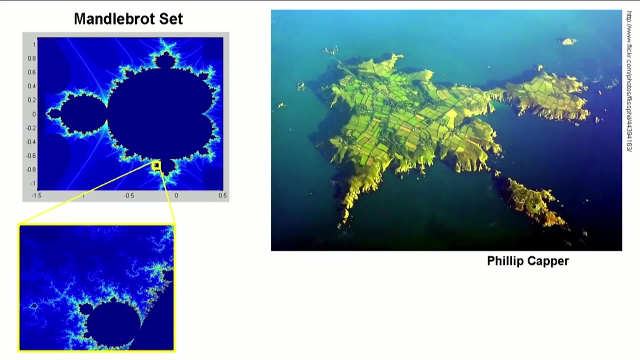 learning it, you start to see it everywhere. People started to see fractals in the geometry of landscapes and close lines like this of Sark, which is in the English Channel. People found uses for fractals in signal and image compression and they even saw fractals. 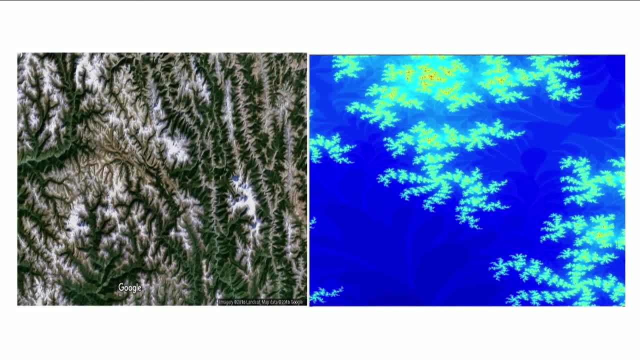 in the snowfall deposits on mountain ridges like this: Google Landsat data on the left and a fractal that I made on the right to kind of mimic the same type of structure and geometric complexity. Fractals even show up in the geometry of the snowflakes themselves and in a staggering 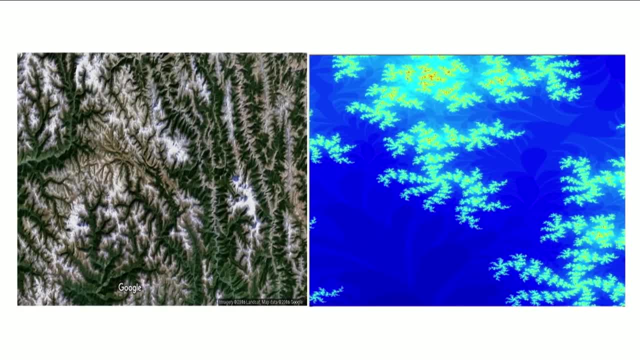 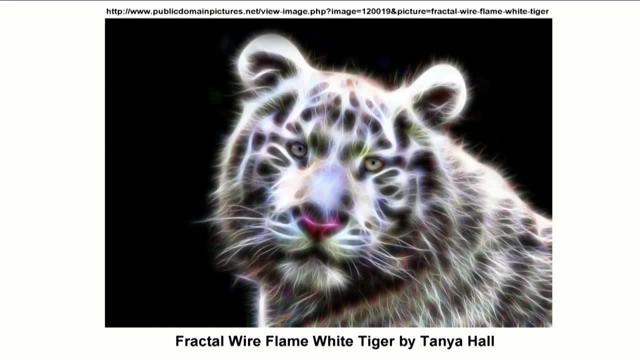 number of biological forms. There are also notable uses of fractals in human creative space, like music and art, where once people became aware of the existence of this type of geometry and they had access to codes with their computer and could make this kind of geometry, they started to make. 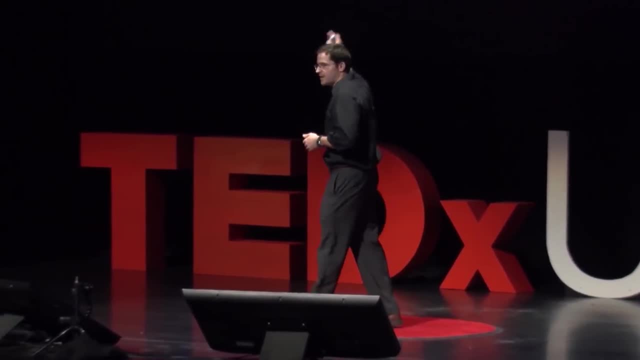 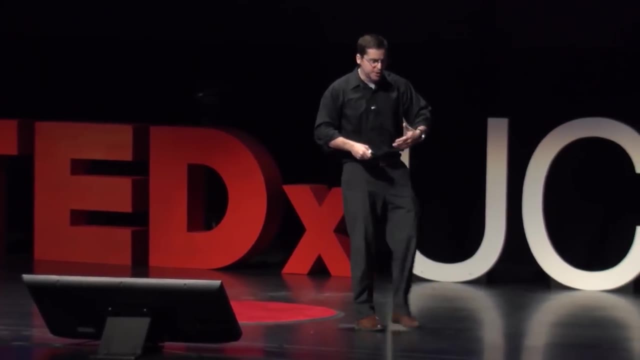 use of it in unpredictable ways. Now, this is an aesthetic application of mathematics, but many people study mathematics just because they find it interesting or aesthetically beautiful. For other people, they want math as a hard skill. They want to be an engineer. 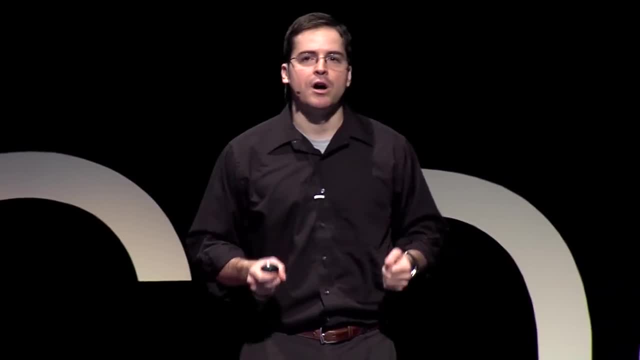 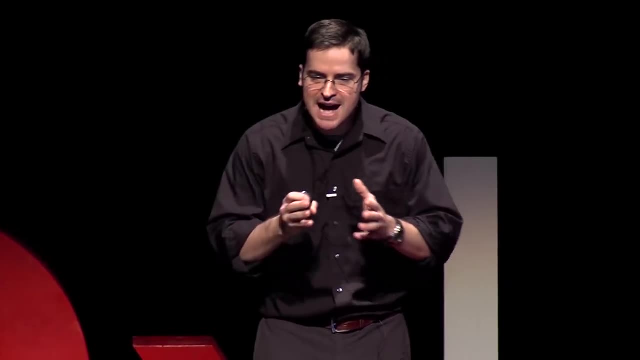 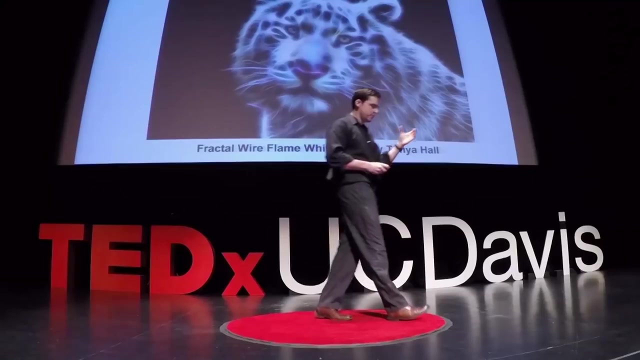 They want to predict the weather, They want to go to space. There is no wrong reason to learn Now. you see, mathematics is like a vast ocean of ideas, The source of truth. And today we took one cup and walked to the water's edge and dipped it in the water and 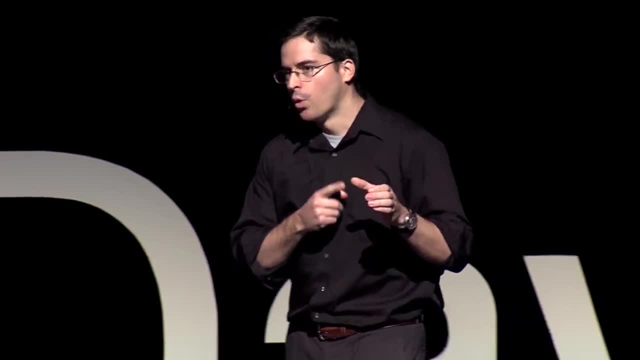 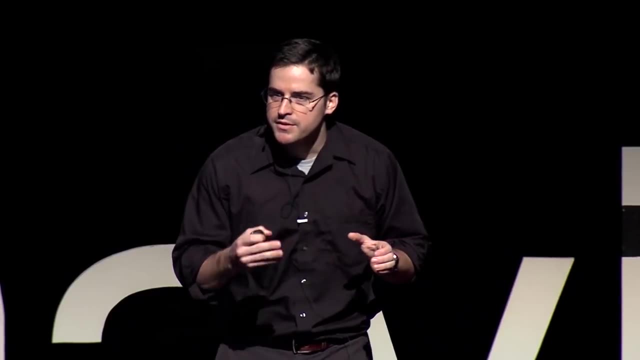 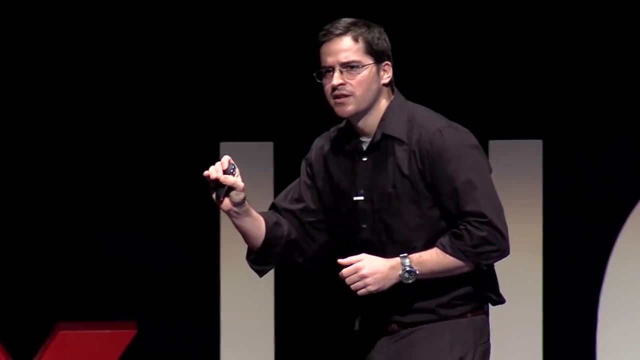 in our cup was one number, pi- One geometric form- the circle- And one equation- Laplace's equation- And just look at the breathtaking scope of ideas that we were able to consider. And finally, in fractals, we just glimpsed the faintest hint of an idea about geometric